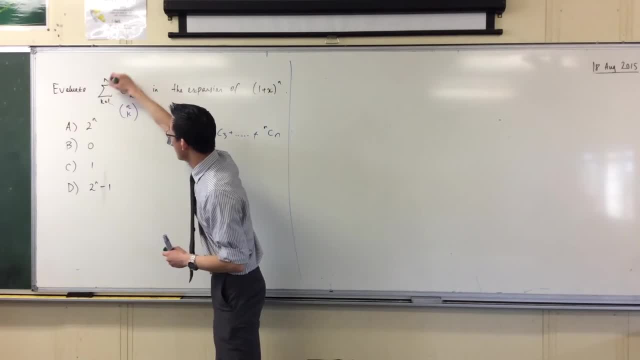 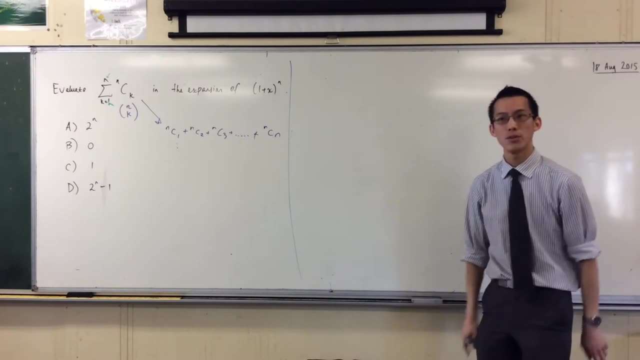 So you've got your first term here and your last term there, So this is what we are trying to evaluate Now. they actually, honestly, they give you an enormous clue, Because this part here on the end is not required to solve the problem. 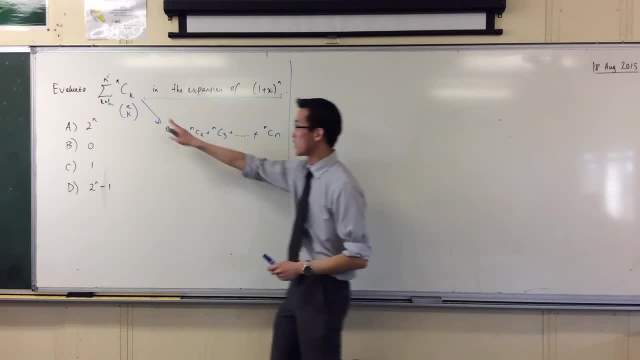 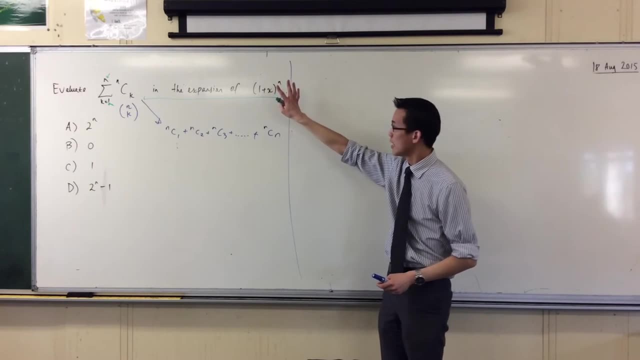 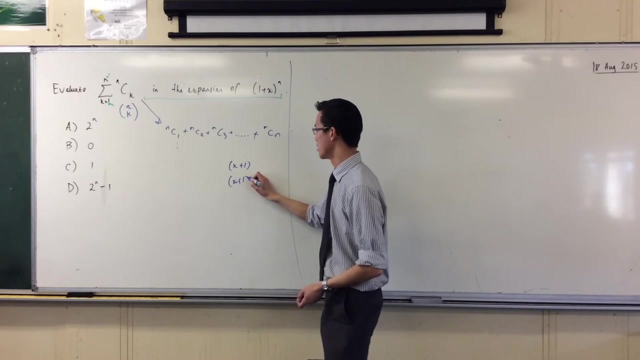 It's them prodding you and saying, hey, remember, remember. the reason why these guys are important is because they appear in the expansion of this. So just to jog your memory, if you think of just a classic example: x plus 1, x plus 1 squared, x plus 1 cubed and 4 would be far enough. 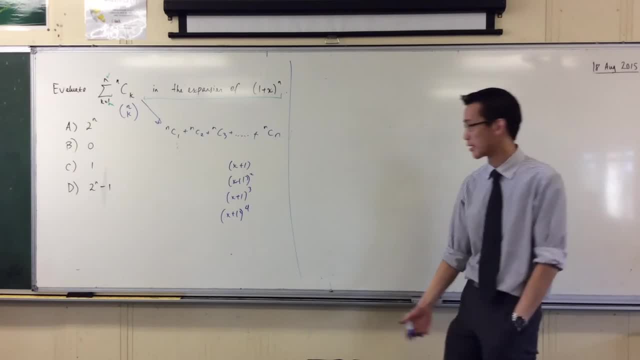 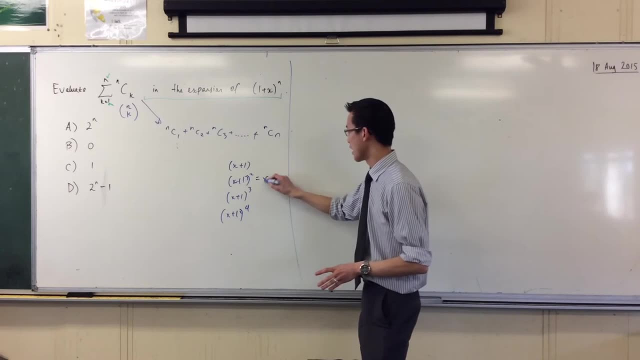 If you just think about your Pascal's Triangle, This is just x plus 1, right? So your coefficients are 1 and 1.. No big deal. When you expand this guy, you get x squared plus 2x plus 1.. 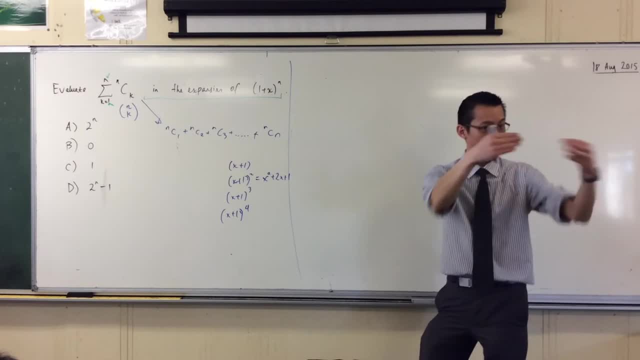 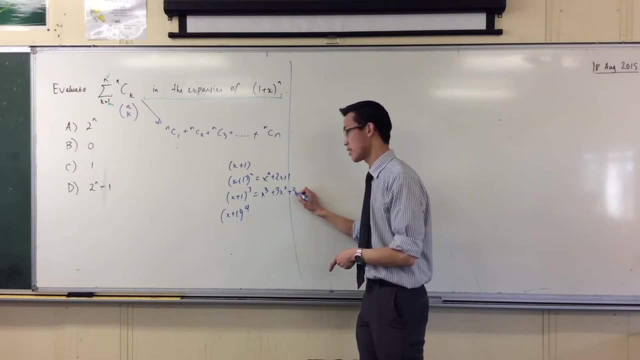 So your coefficients are 1,, 2,, 1.. You go down to the next row. help me out. Yep, there's the 1, there's the 3,, there's another 3, and then there's the 1 trailing on the end. 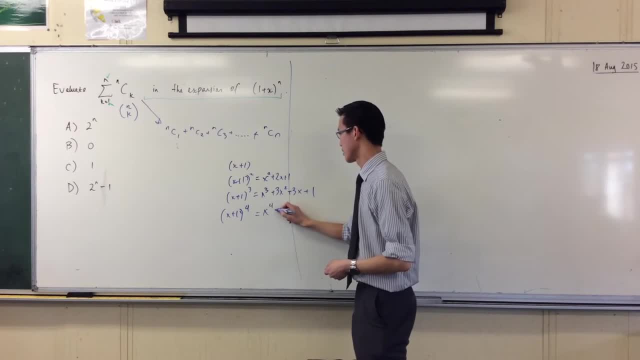 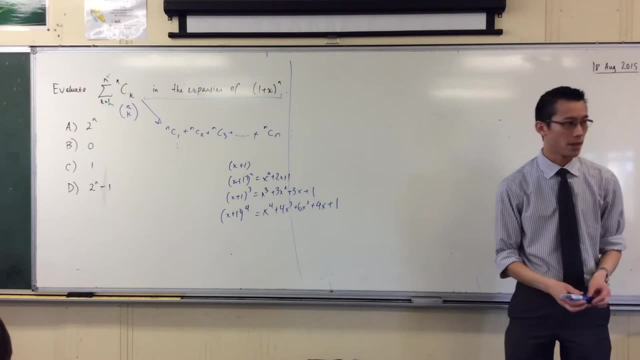 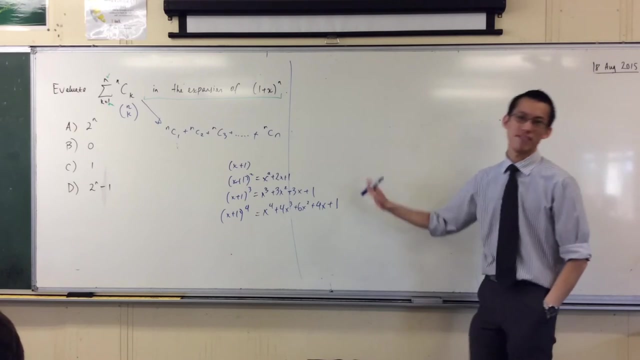 And if you go one more row down, you're going to get 4, 6, back to 4, because it's symmetrical, remember, And we finish with 1.. Doesn't take you much to go and do, that'll be 1, 5, 10, 10, 5, 1, etc. 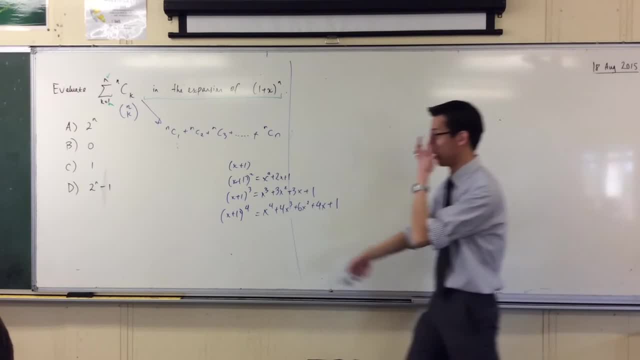 You don't tend to see them very often, unless it's some multi-part question. This is multiple choice, so that's why they kind of just leave it open. Now, being that you can see this pattern forming. when they give you something like this, it's like: oh, I don't know where it's going to end. 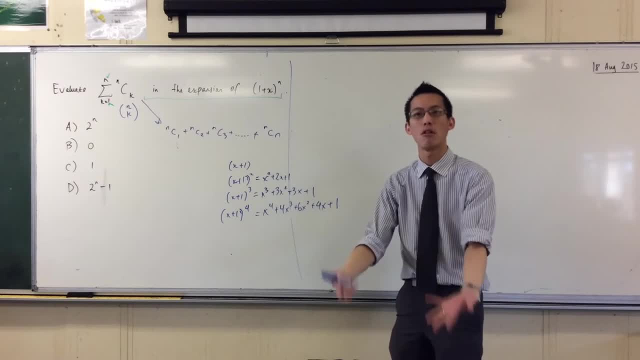 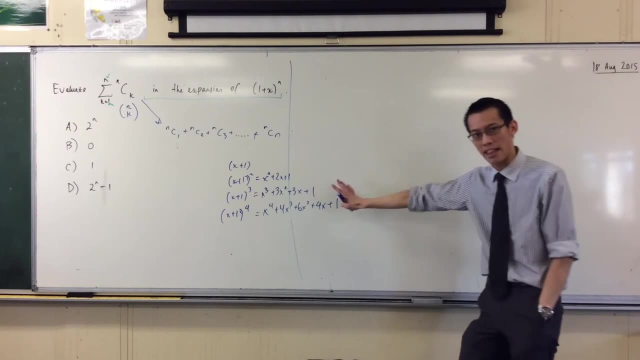 That's one of the strategies we use to make things happen. It's harder, right? It's introducing more algebra. If I just said 3,, just go up to 3, that would be easy. You don't need to really apply that much thought. 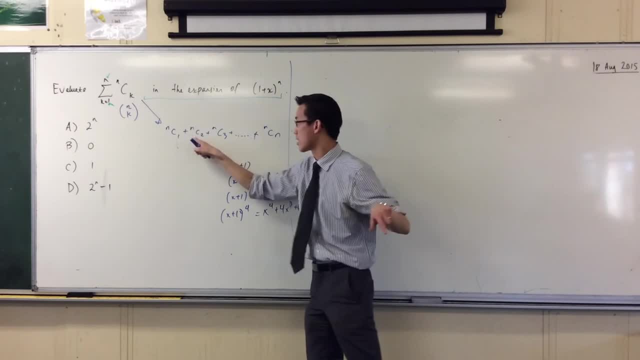 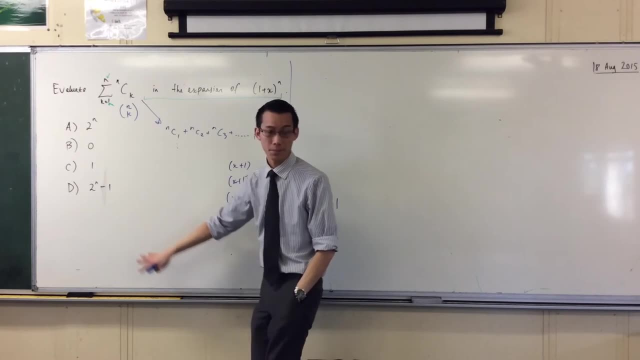 You just go up to 3, you add them all up. these guys correspond to these coefficients, and now pops your number. So the fact is, algebraic is a bit harder. Now have a look with me These coefficients that are written in there. 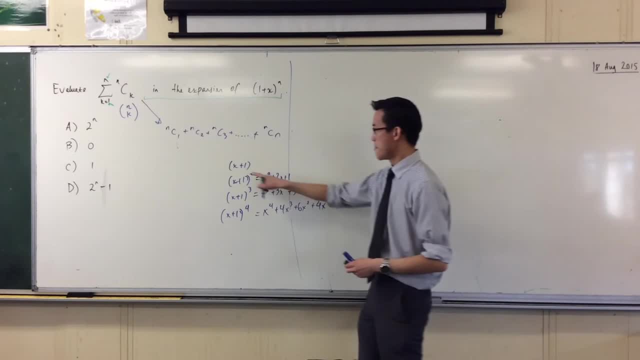 I'm actually just going to write the coefficients out, Right? This is the. which row of Pascal's triangle is this? It's the? it's a bit funny, right? It's row number 2, if you're just counting 1,, 2,, 3,, 4,. 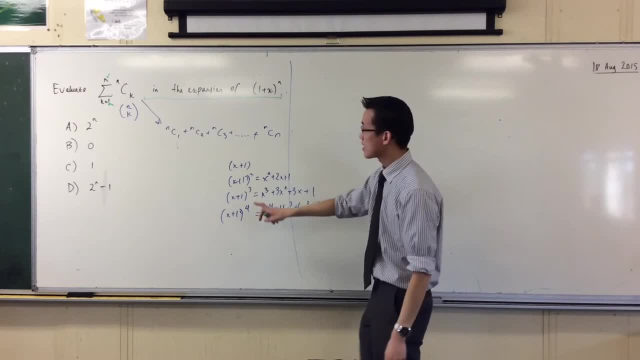 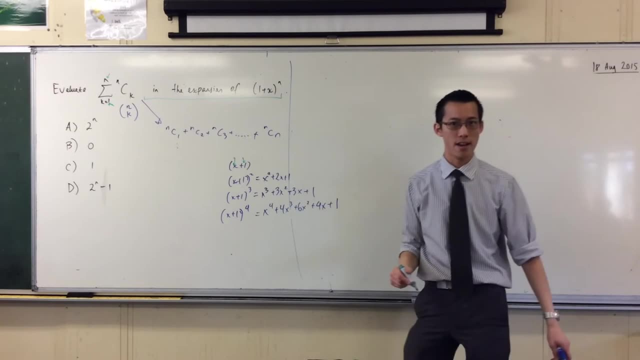 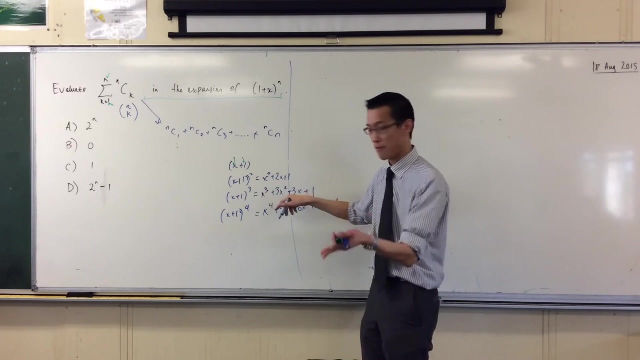 but it's actually. it is the first row, right. It's for n equals 1, okay, So what are the actual coefficients that give me 1 and 1?? Now, by using this NCR notation, right, you may remember. 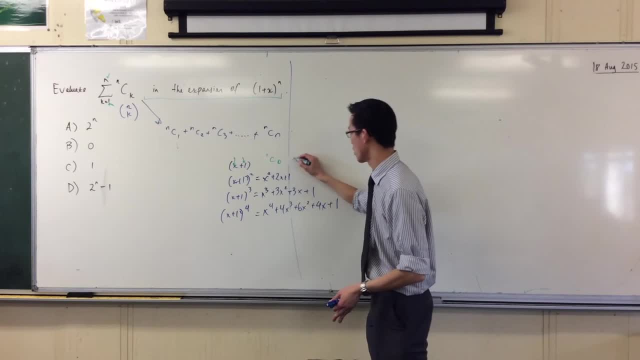 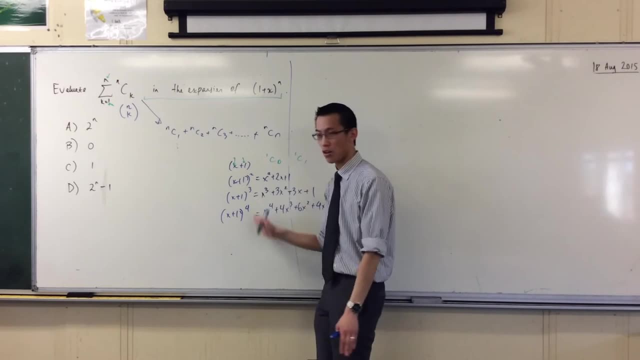 we call them 1C1, sorry, 1C0 and 1C1, okay, It's a bit weird, isn't it, to say you're choosing nothing, but that's why these N terms are always 1,. 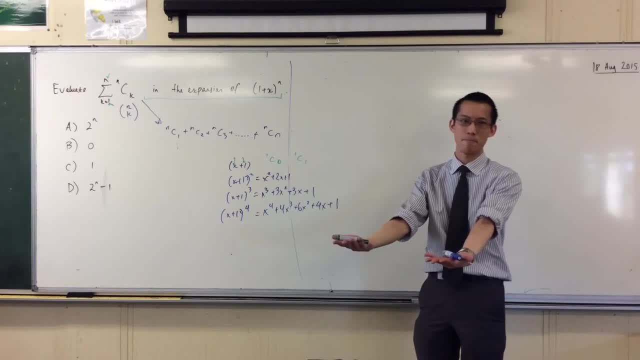 because how many ways are there to choose none of my whiteboard markers? And the answer is: there's one way to choose none of them. No matter how many whiteboard markers you're holding, there's one way to choose none of them. 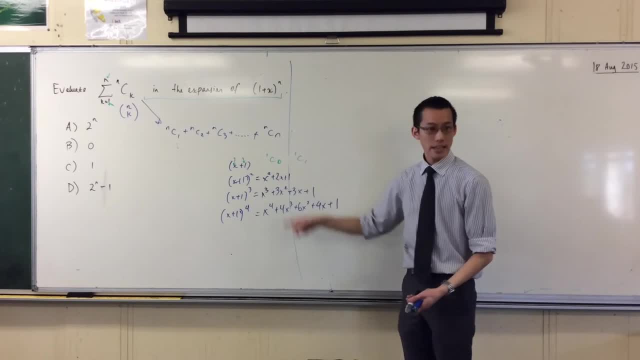 So all of the first ones are called 1C0? Well, they're called whatever. C0, right? So this number on the top is which row you're on, Okay? So then, when we go to the next one, you're going 2C0,, 2C1,, 2C2, right. 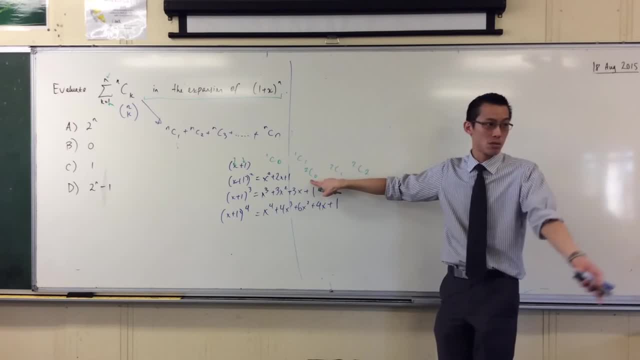 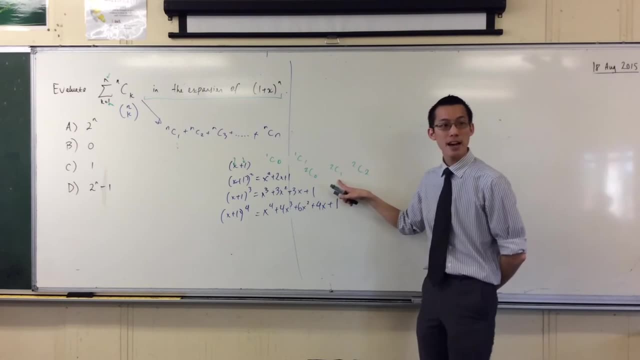 There's only one way to choose none out of two. There's only one way to choose two out of two. right, If you only can choose two? And how many ways are there, if you've got two to choose from, to pick one of them? 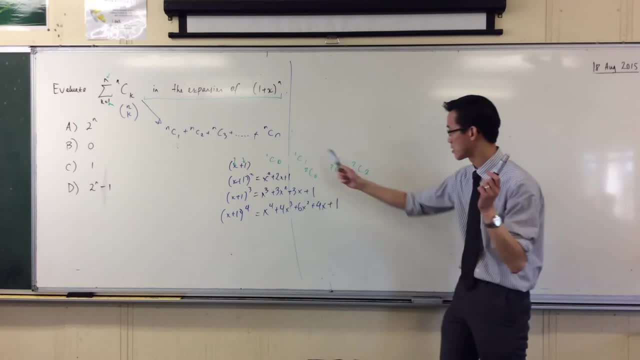 Answer: one way, two ways right, Hence two. okay, Now you can see the pattern that's forming right. So you've got. sorry. this is the third row: 3C0, 3C1, 3C2, 3C3.. 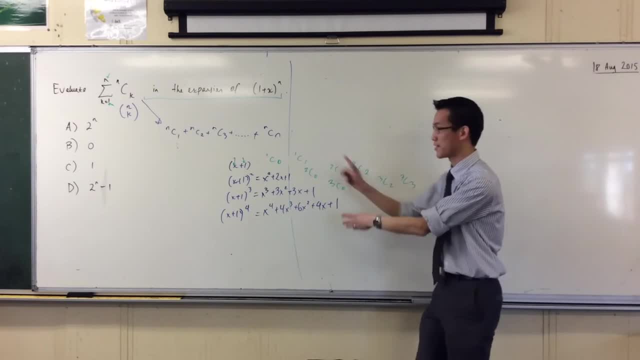 Okay, you're getting the idea. Now, how this relates to this is: they want a sum, They want a particular sum. okay, So let's try and follow this pattern and see what's going on. right, When I add up these guys, that's just one plus one. 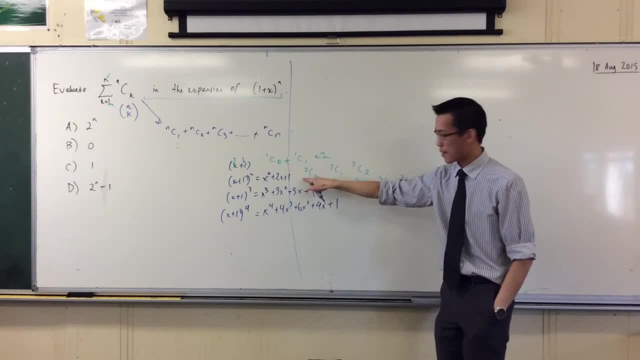 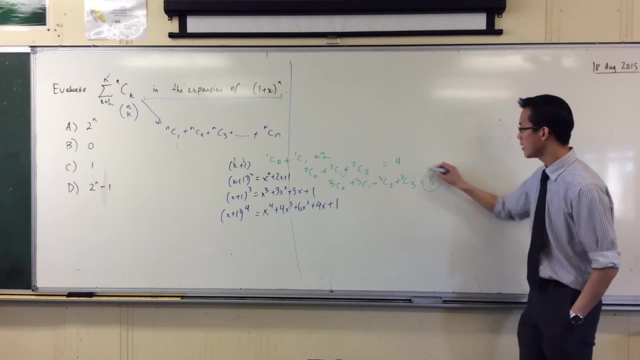 Two, no big deal. When I add up these guys, I'm adding one plus two plus one, which is four. And then when I add up these guys, I'm doing one plus three plus three plus one, which is eight. So the pattern has formed okay. 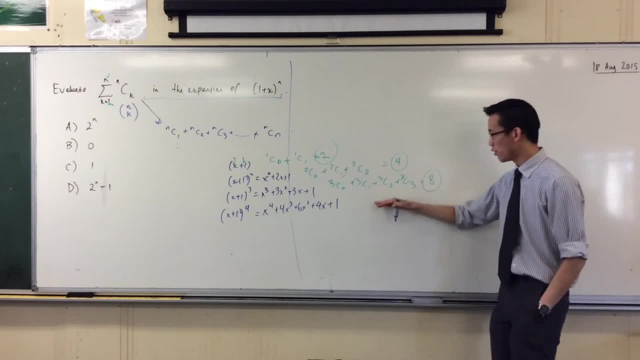 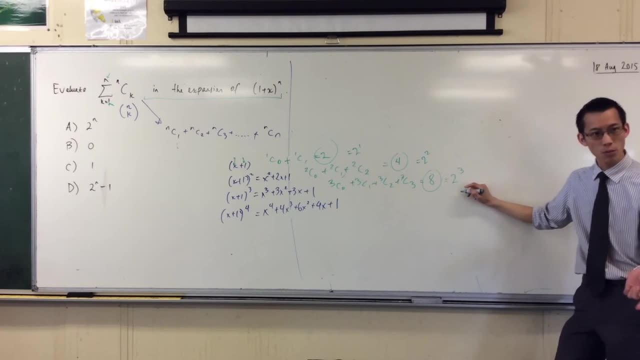 You see the pattern. Okay. Now, therefore, you can rewrite these numbers as two to the one, two squared, two cubed. In other words, it's two to the n. if, if, careful, I'm not at the answer yet. 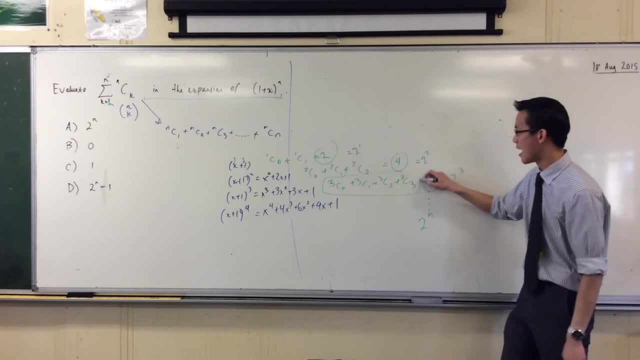 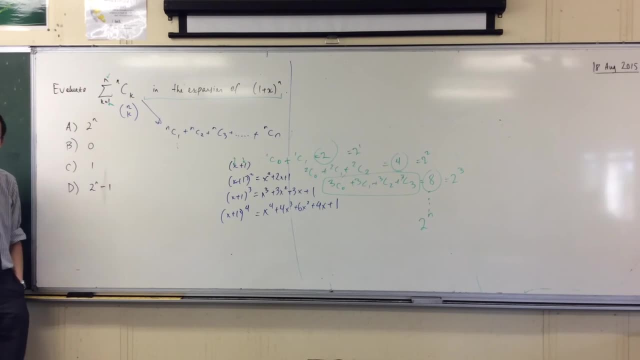 It's two to the n. if I add up all of the items, all of the items in the row, Does that make sense? I've got to add them all up. okay, Now look carefully at the question. Read carefully. Is the question asking me to add up all the terms in the row? 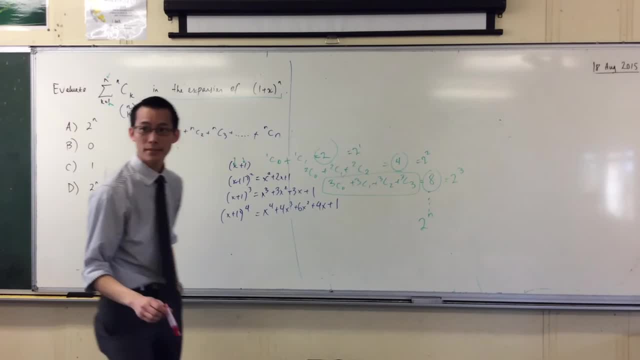 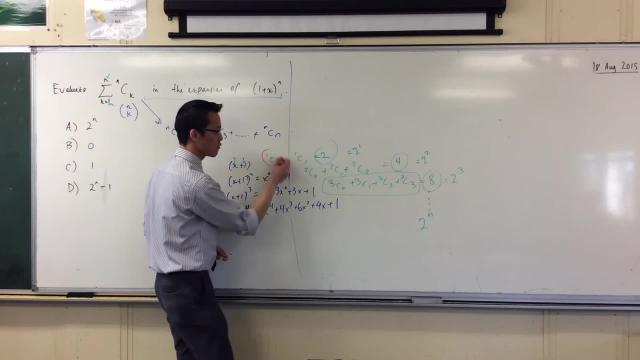 I don't even know what it's asking you And the answer is: it's missing one. Look, I wrote it out here, right And see: one, two, three, four, all the way up to eight: zero. I'm missing zero every time. 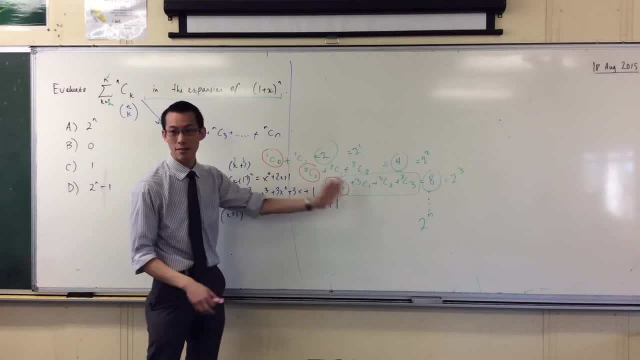 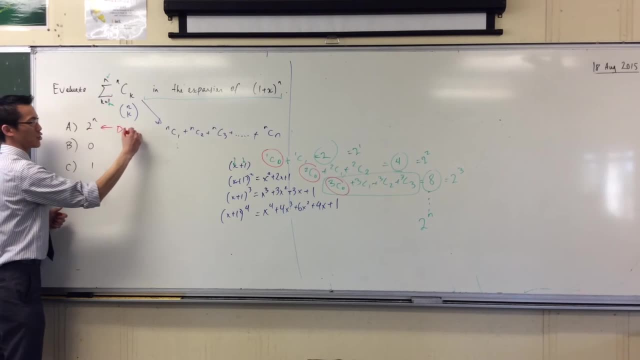 Okay, The first time, the first term in each row is always one, Right? So therefore I'm not two to the n. We call this a distractor. Yes, Right, I'm actually not kidding. Multiple choice question design is a big deal. 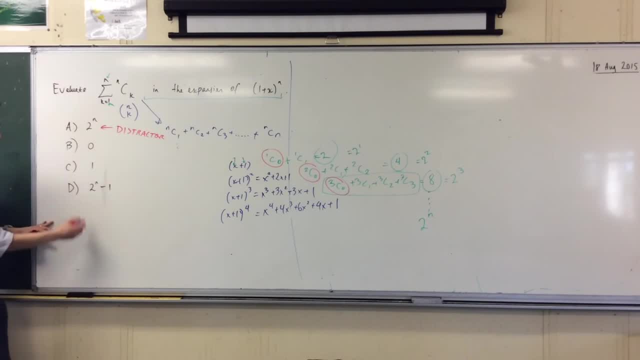 and they're called distractors Because you think about this, right? So you can see, here's the answer, right? If this was the actual answer and all the rest of the answers were like you know, I don't know, like minus one and 256 and 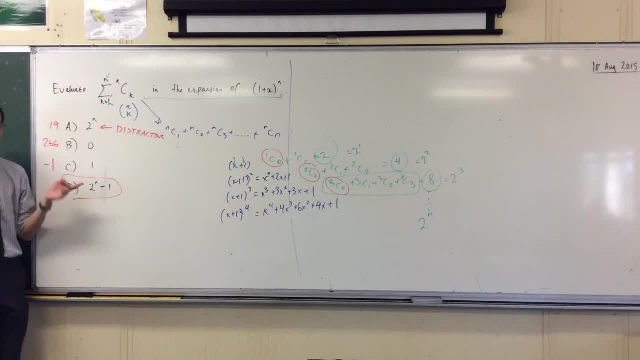 There's two of them that are obviously one, Nineteen. okay, Then you're like: well, I don't know, They're obviously one. If you take a different approach to doing this, you can plausibly end up with zero and one, which are also equal. 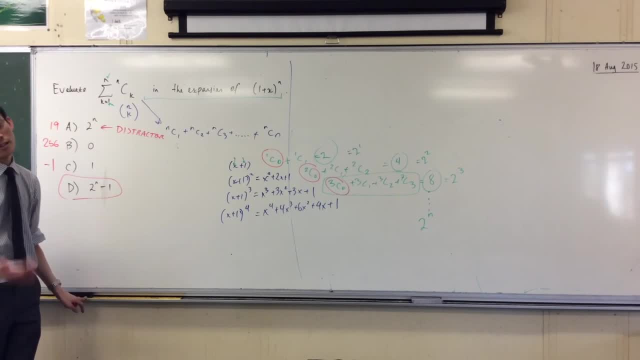 But there's always two which are going to be like the same, but one thing different, and you know it's going to be one of them, That's true. So, anyway, this is the better distractor, as you can see. Okay, It's even put up the top of the question to troll you even further. 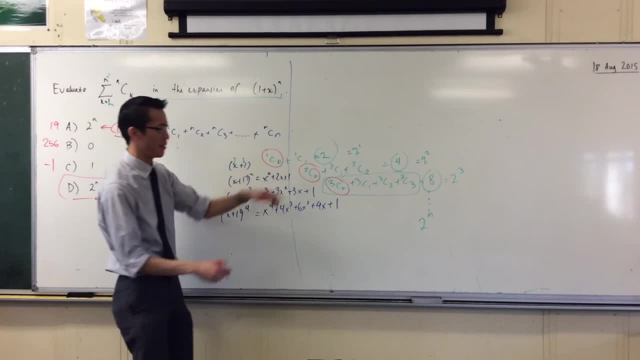 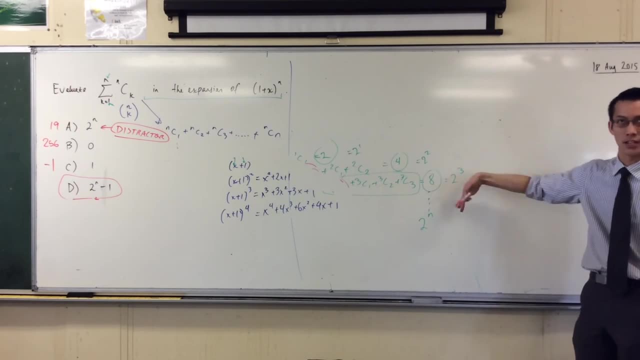 Okay, This is really what they're doing, because every time, if we wipe all these guys off, you're always one short. You won't have two, four, eight. You'll have one, three, seven, fifteen, etc. Okay. 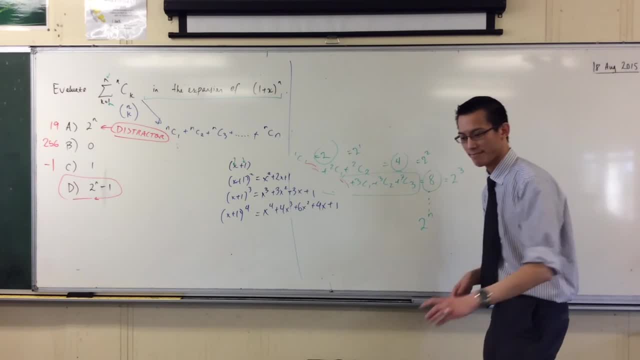 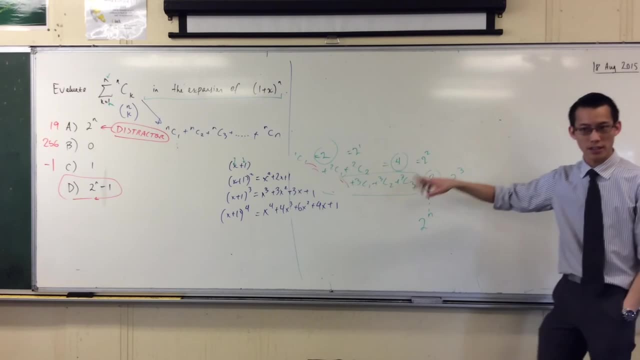 Yeah, Also, every single time that you take the first term, the first term is always one, Correct. Therefore, you take one off. That's exactly right, Yeah, One C naught. two C naught. three C naught. anything C naught.